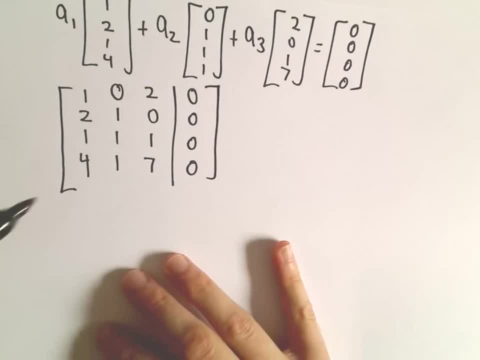 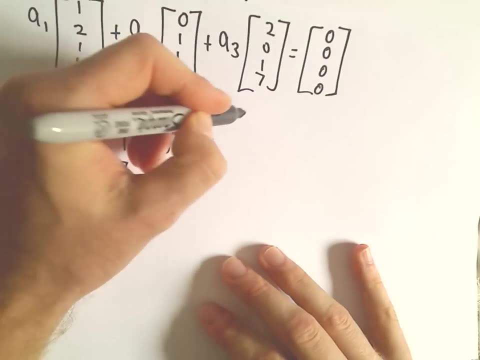 So a little more tedious, but hopefully it won't be too bad. So I'm going to do negative 2 times the first row and add that to the second row to get my new second row Again. this is the type of stuff that is very useful to have a calculator for. 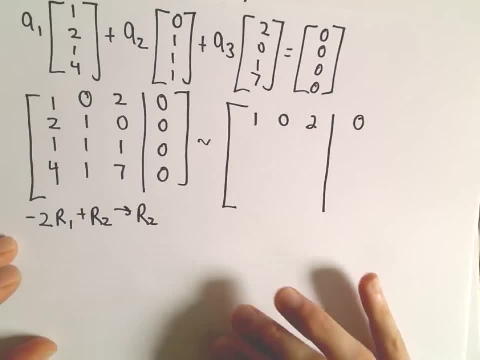 But again you may have to do it by hand in class, So let's do it this way. So negative 2 times 1 plus 2 is 0.. Negative 2 times 0 plus 1 is 1.. Negative 2 times 2 plus 0 is negative 4.. 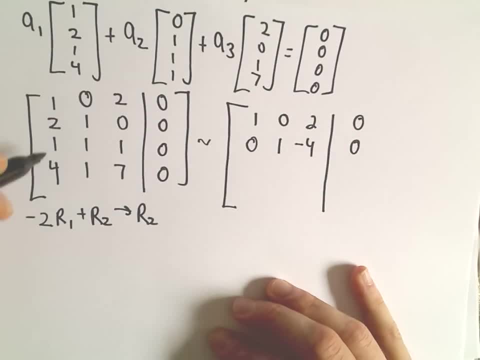 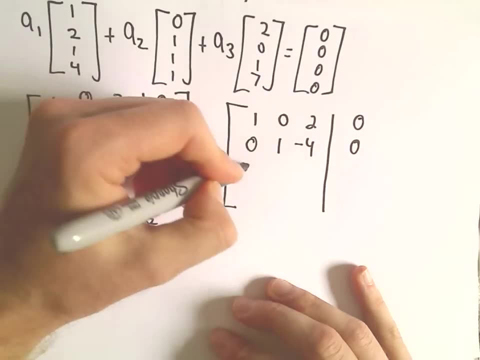 And then we'll just get 0. Always 0s. in the last, We can do negative 1 times row 1, add that to row 3 to get my new row 3. So we'll get negative 1 plus 1, which is 0.. 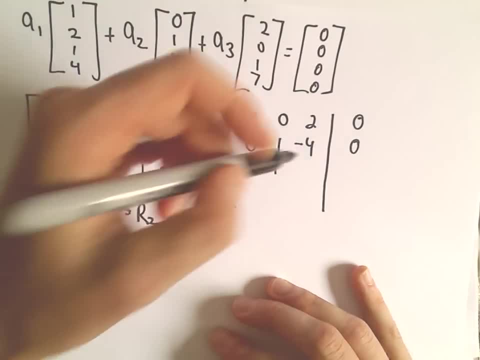 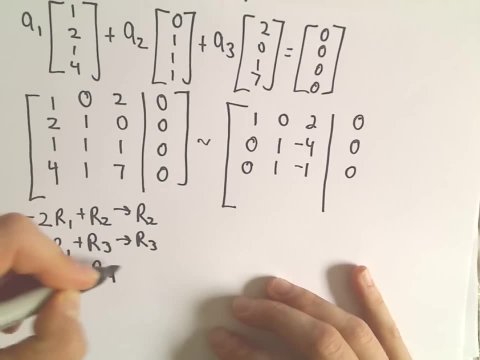 0 plus 1, which is 1. We'll get negative 2 plus 1,, which is negative 1.. And again a 0. Then I think we can do negative 4 times row 1 to get my new row 4.. 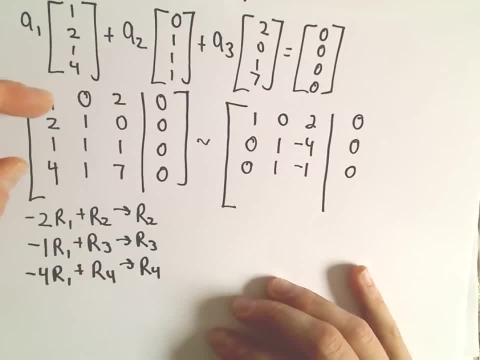 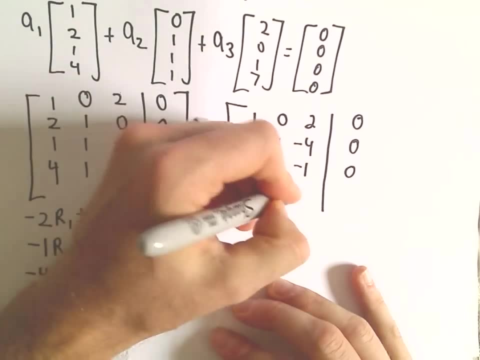 So negative 4 times row 1 plus row 4 to get our new row 4.. So negative 4 plus 4 is 0.. 0 plus 1 is 1.. Let's see We'll get negative 8 plus 7, again, which is negative 1.. 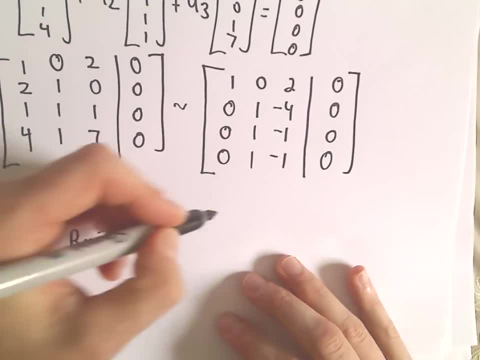 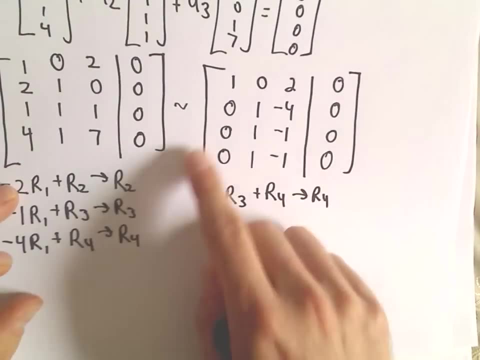 And then some 0s Notice immediately. we can do, for example, negative 1 times row 3 and add that to row 4 to get my new row 4.. I'm basically noticing that they're exactly the same. So if I just multiply one of those by negative 1 and add it to the other, 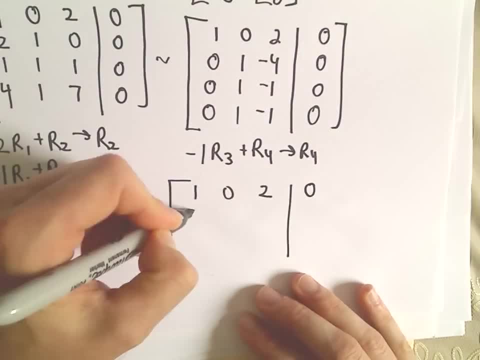 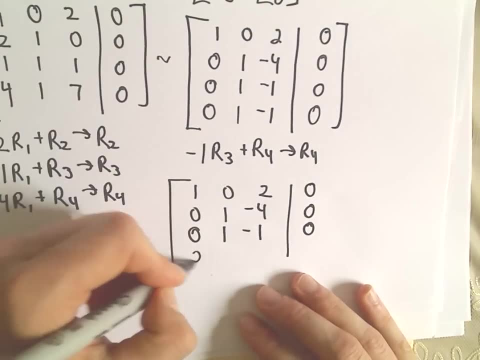 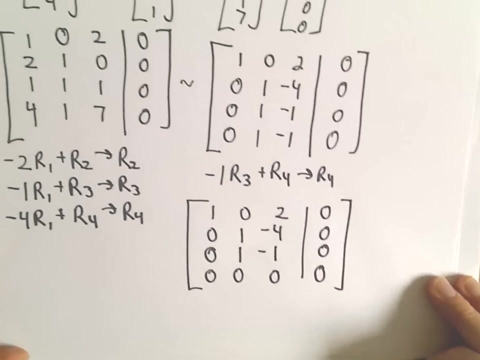 we can simply make that row into a bunch of 0s- 0s- Okay, So if we do that, that's going to make the last row into 0s. Now you might think, just because we have this row of 0s again, we have non-trivial solutions. 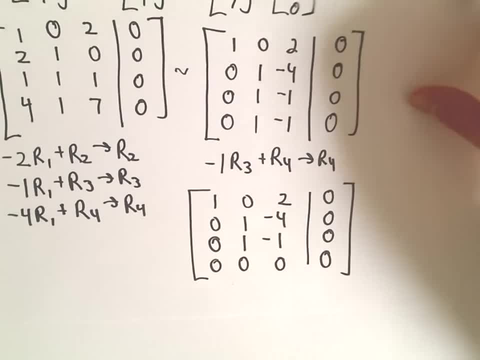 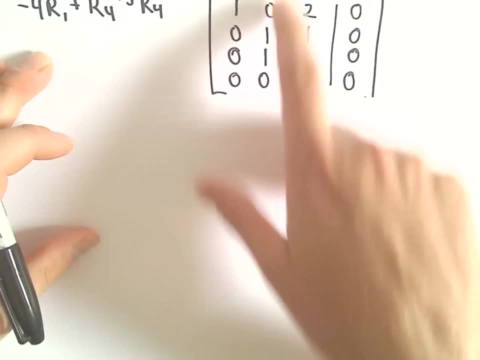 But let's keep going just to make sure here, because in fact that's not correct. So let's see here. So we've got our 1 in our second row, second column. That's good. So we can do negative 1 times row 2 and add that to row 4.. 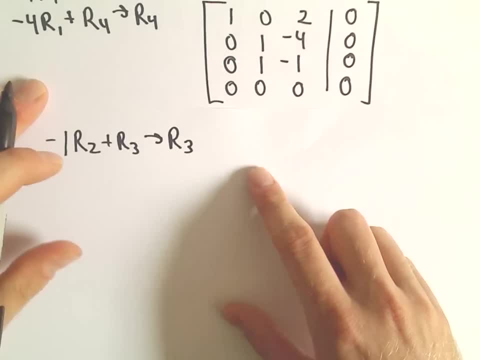 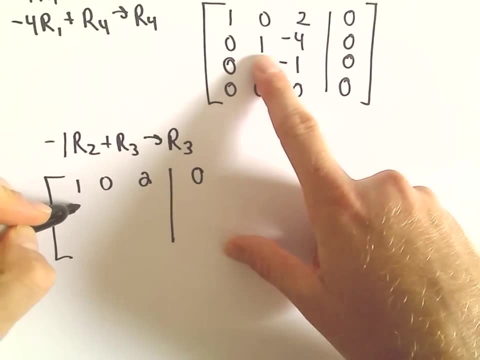 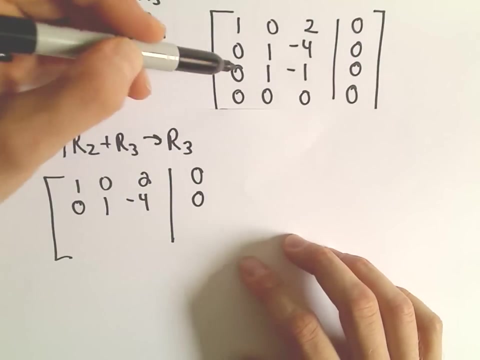 So I'm going to leave the first row alone: 1, 0,, 2, 0.. I'm going to leave the second row alone as well. So let's see, If we multiply it by negative 1, we'll just get 0.. 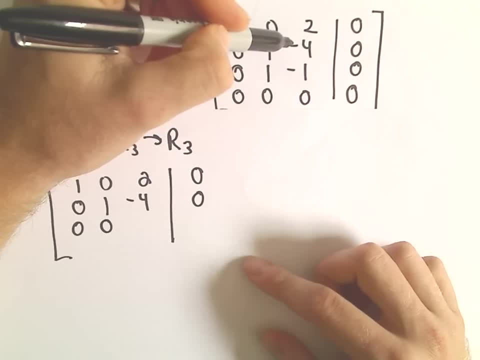 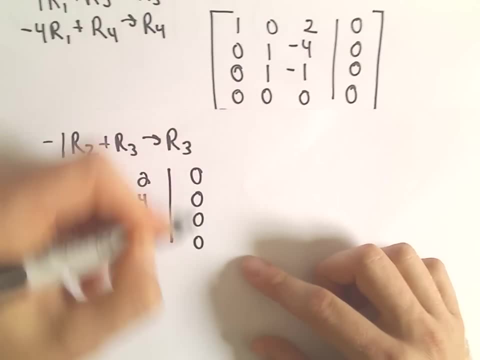 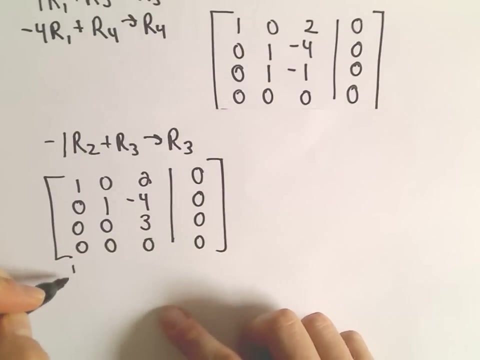 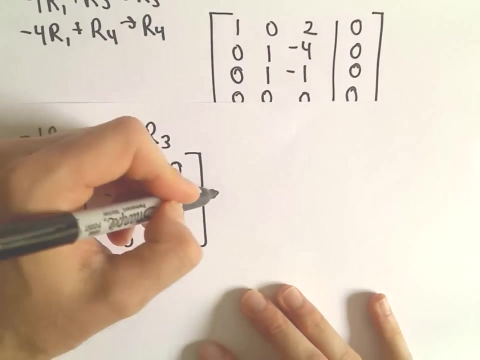 Negative, 1 plus 1 is 0.. We'll get, let's see, I guess, positive 4 minus 1, which is 3.. And then we still have 0, 0,, 0, 0.. We can take our third row and just divide that by 3 to make that third row, third column, into a 1.. 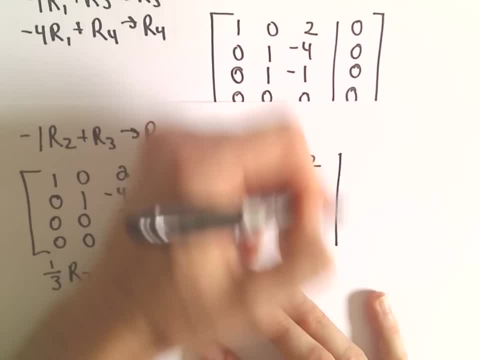 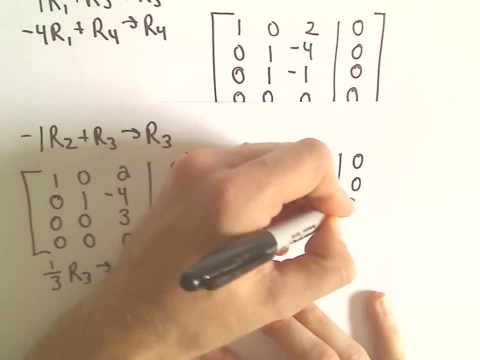 So 1, 0, 2, 0, 0, 1, negative 4, 0, 0, 0, 1, 0, 0, 0, 0, 0.. We're having fun. 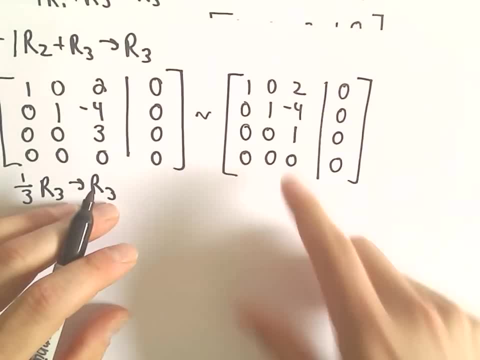 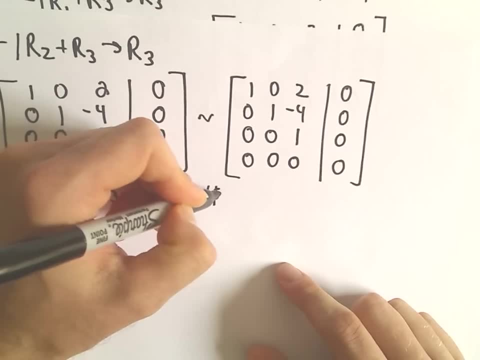 And notice now what's going to happen is we can basically just zero out the rest of the entries in the third column. So if we do 4,, well I guess let's do negative 2 times row 3 and add that to row 1 to get our new row 1.. 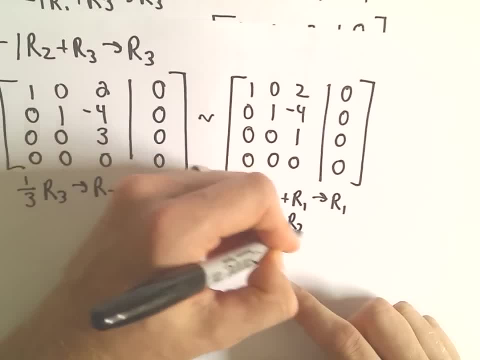 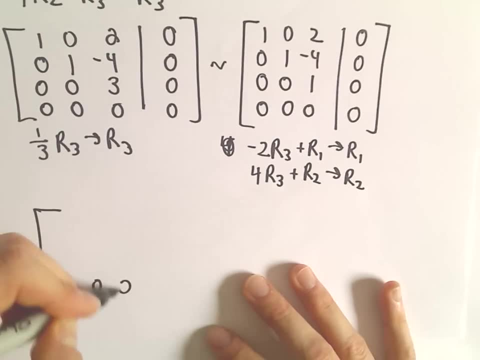 And then we'll do 4 times row 3, add that to row 2 to get our new row 2.. So again the bottom row 0, 0, 0.. The third row we're leaving alone. 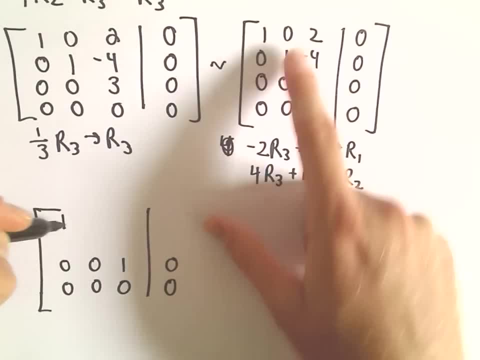 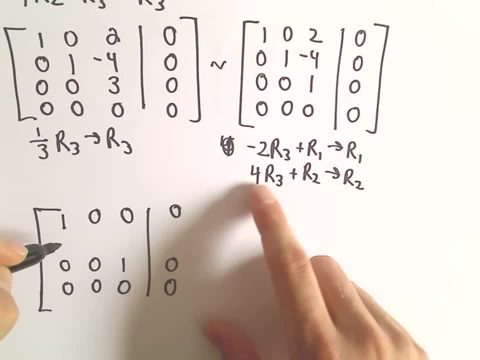 If we take negative 2 times the third row, we'll be left with 1, 0. We'll have negative 2 plus 2, which is 0. Again, 0. We've got. if we do 4 times row 3 and add that to row 2, we'll get 0, 1.. 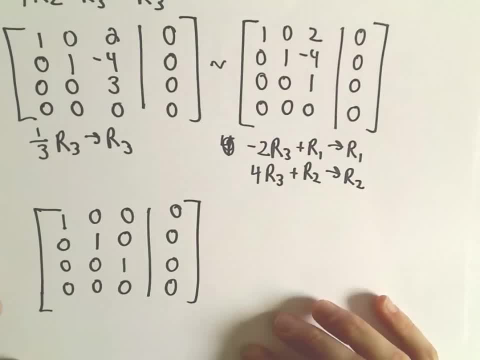 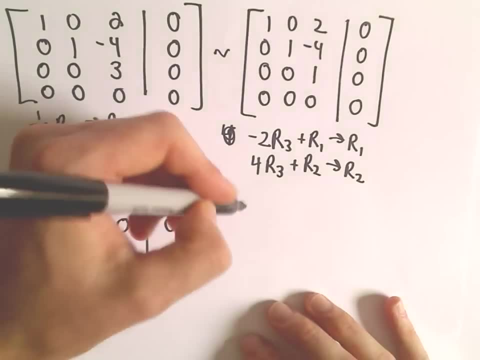 And then that'll make that into a 0 and a 0.. So now this tells us: you know again, these were the values of our scalars: a1,, a2, a3.. The first row says: well, a1 has to equal 0.. 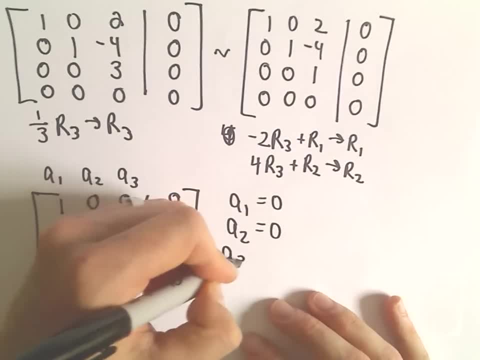 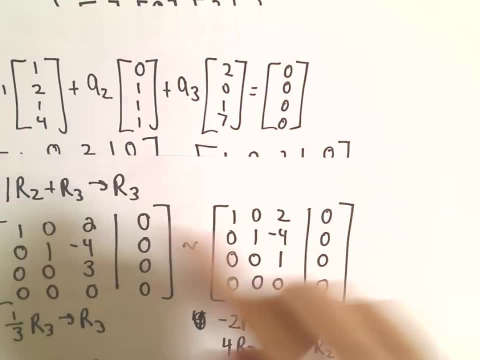 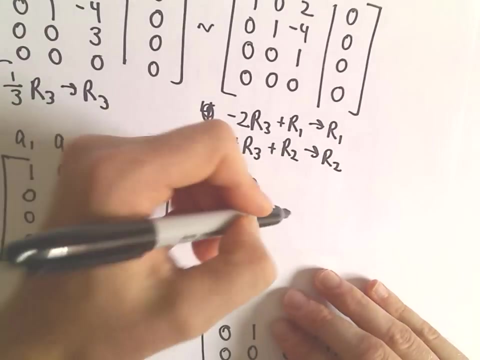 It says a2 has to equal 0. And the third row tells us that a3 also has to equal 0 for that original equation to be satisfied. So it says the only way this original equation is satisfied is if a1, a2, a3 all equal 0..